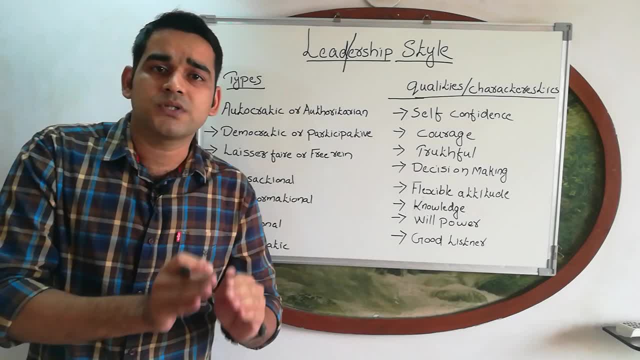 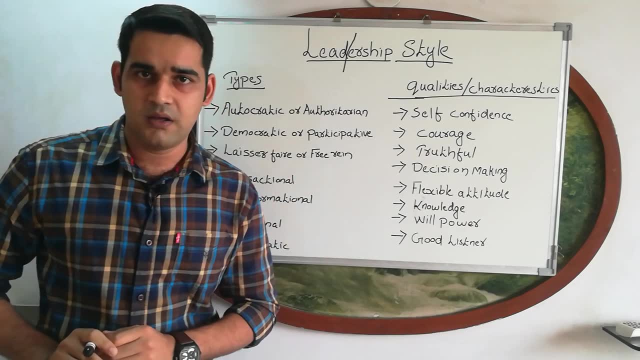 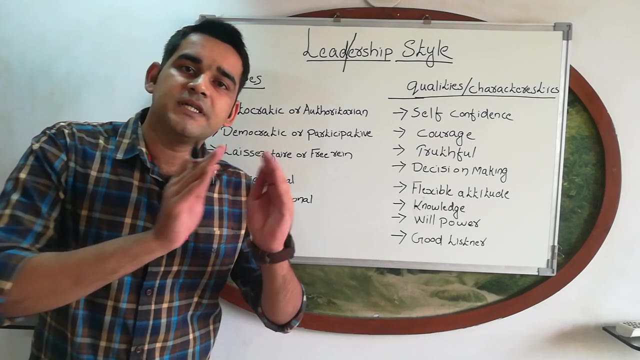 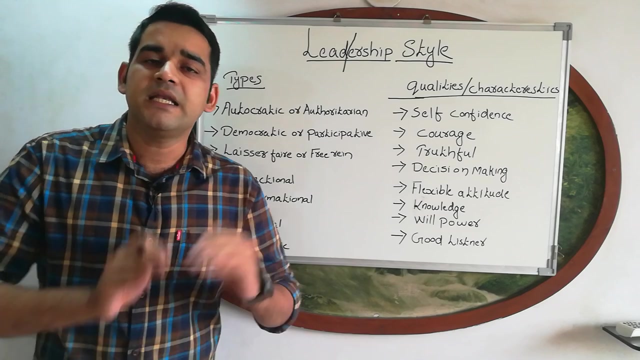 individual by sorry. it is a process of an individual is influencing a group of individuals to achieve the common goal. an individual is influencing a group of individuals- okay, a person is influencing a group of peoples for what? to achieve the common goal. so you can define leadership as it is the process. 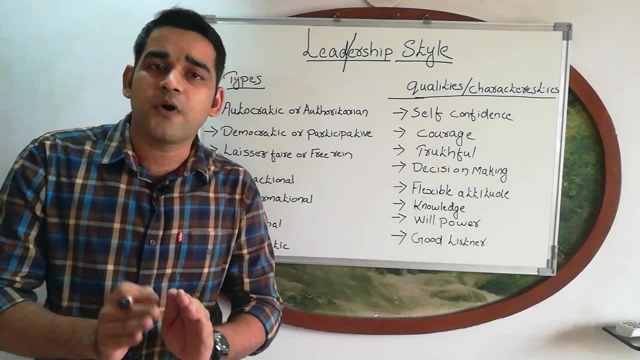 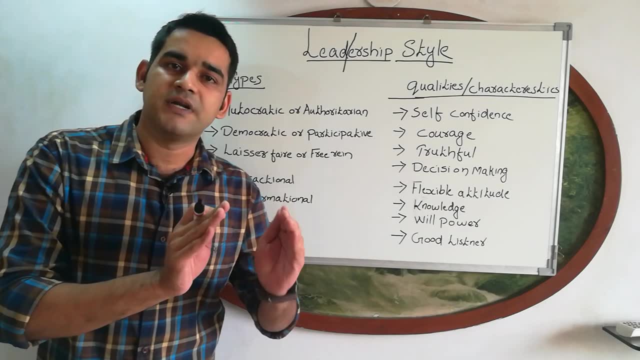 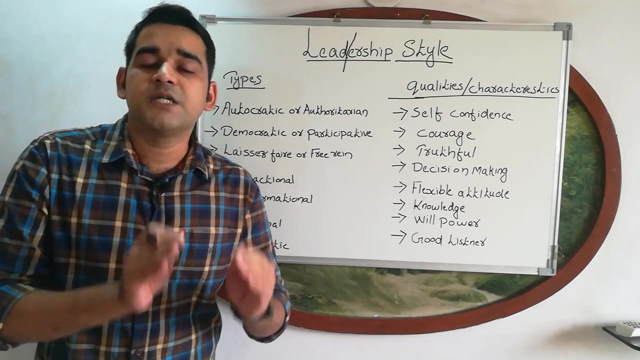 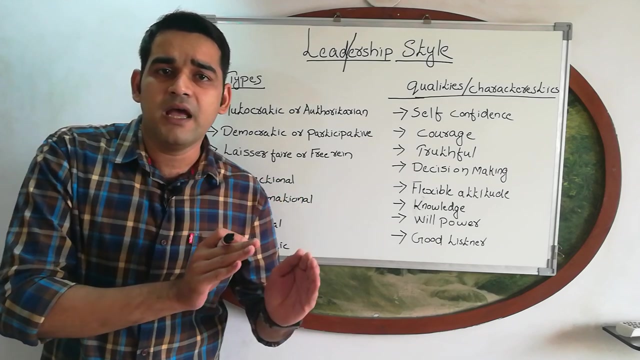 of an individual is influencing a group of individuals to achieve the common goal. to achieve a thing, a person is influencing a group of peoples. that is leadership. what it next we can see: leadership style. what is leadership style? leadership style is nothing. it is the different way to implement the planet. 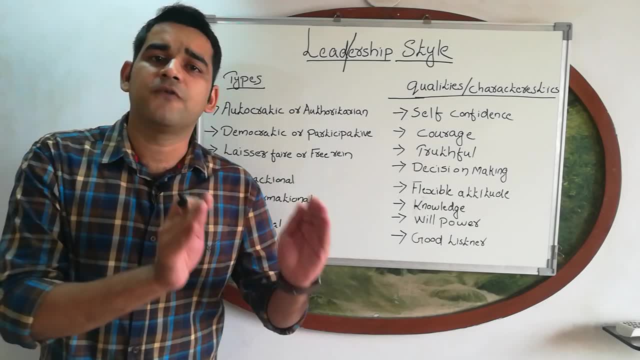 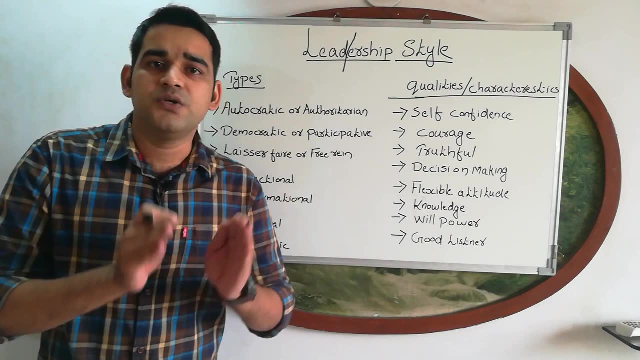 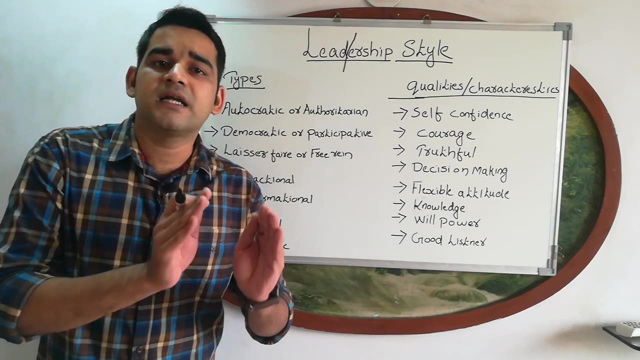 okay, so for the leader, he have to influence a group of peoples. so the different ways or the different techniques used to implement the plan to achieve the goal, that different techniques are used, that is leadership style. so you can tell leadership style as it is, the way it is the. 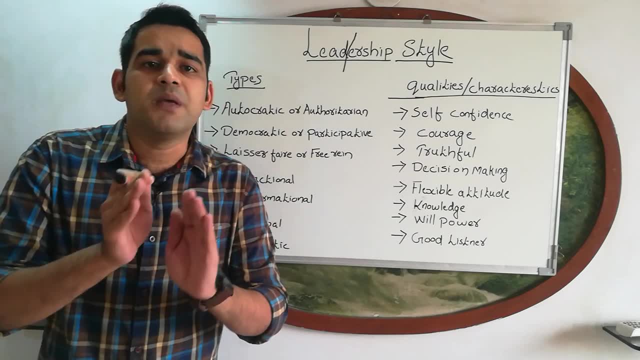 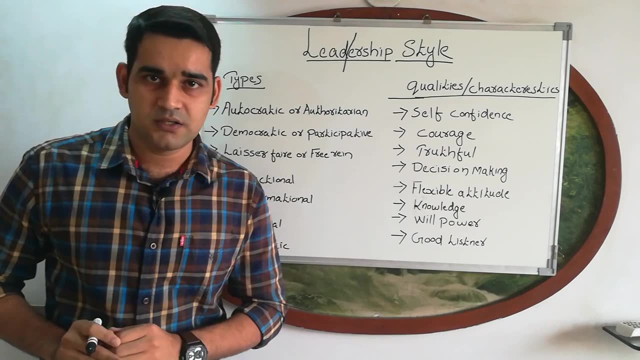 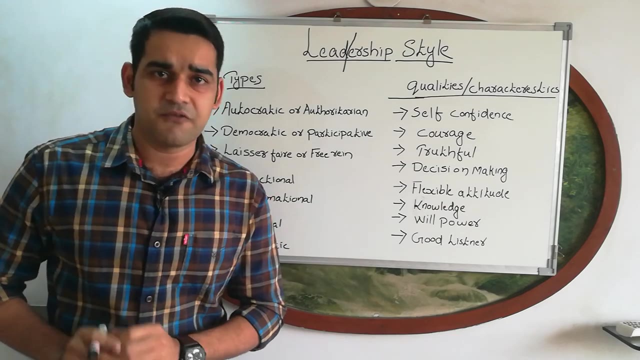 way used by the leader to implement the plan got it. next we can see the different types of leadership styles. you can see different different types of leadership style. most important one i am discussing here. we can see one by one. first one is autocratic or authoritarian leadership. 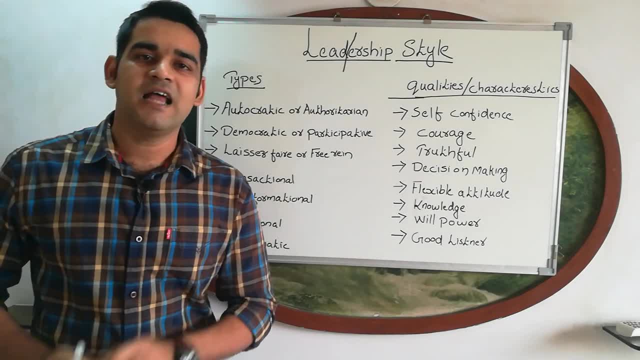 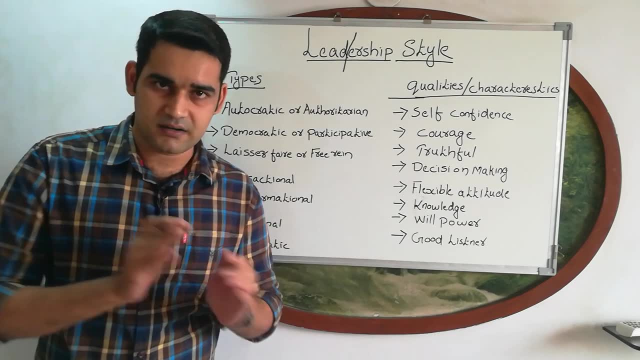 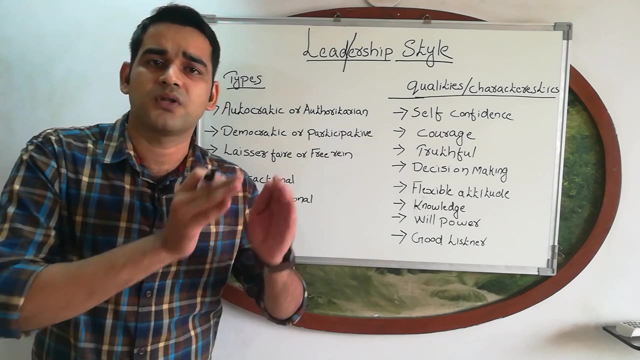 style, autocratic or authoritarian leadership style. that means all the decisions and all the plans are done by the leader and he is just giving the order or he is just giving the command to the subordinate or to the workers to follow that. simply you can say that all the decisions and 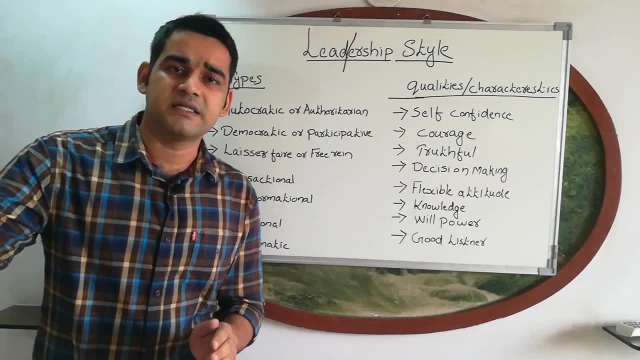 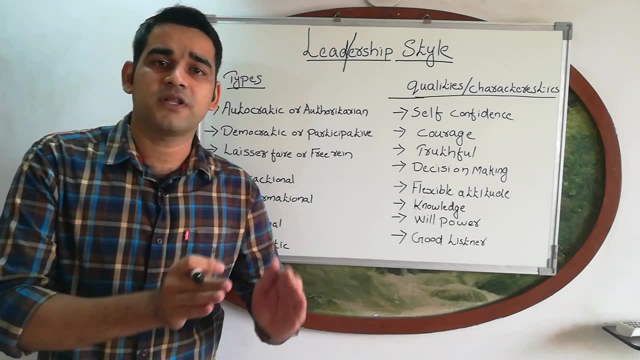 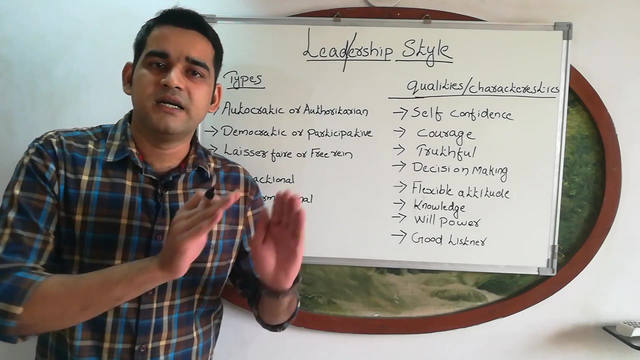 plans are taken by the leader and he is giving that instruction to the workers to follow that the workers should follow that. there is no role for the workers. the role of the subordinate or the worker is just follow it. okay, all the decisions and the plans are made by the leader, only that is. 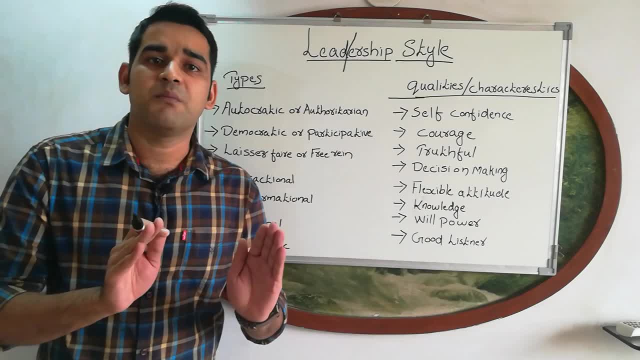 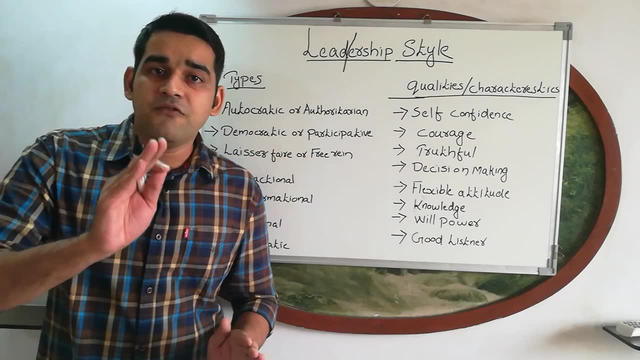 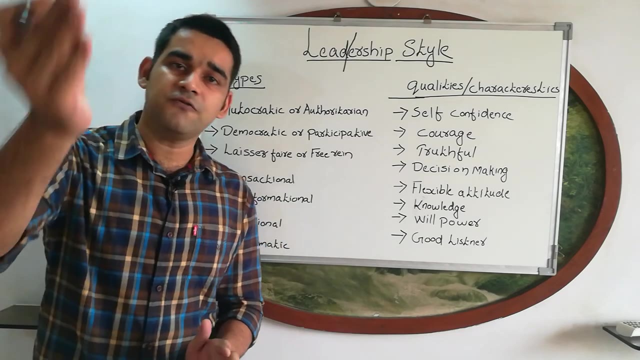 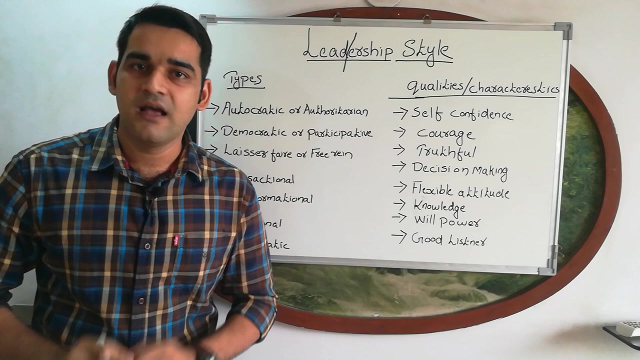 autocratic or authoritarian. for example, adolf hitler was a autocratic leader. okay, so simply you can say that i will decide and you should follow. that is autocratic leader leadership. the leader will decide and you should follow that is, the workers or the subordinate should follow that. that is autocratic or authoritarian leadership. okay, next one is: 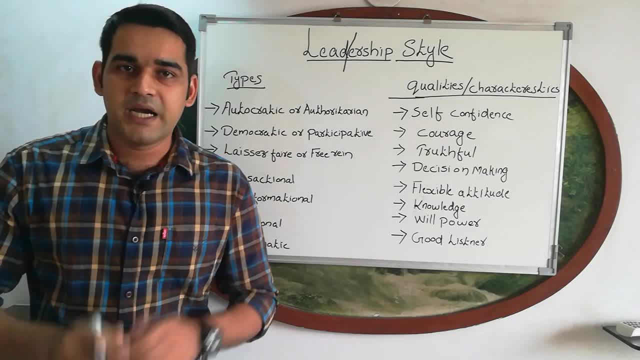 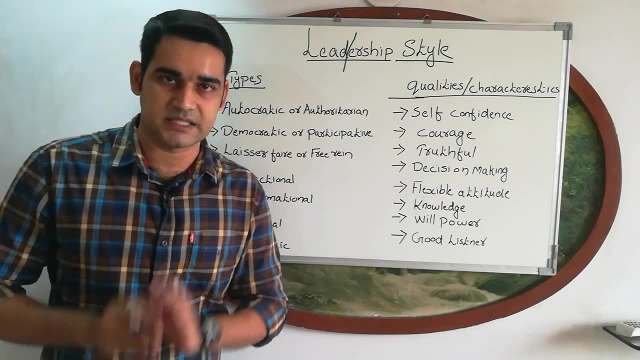 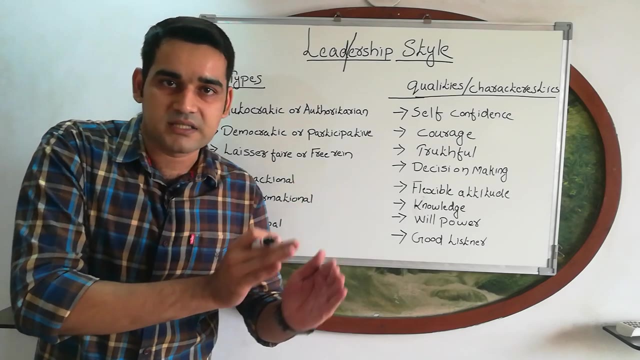 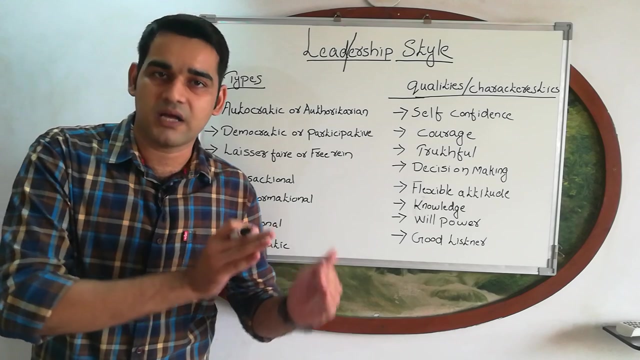 democratic or participative leadership. democratic or participative leadership: that means just opposite to autocratic. that is, all the decision and the plans are done by the leader, as well as the subordinate or the workers. They will togetherly, they will decide and they will togetherly will plan the things regarding the organization. 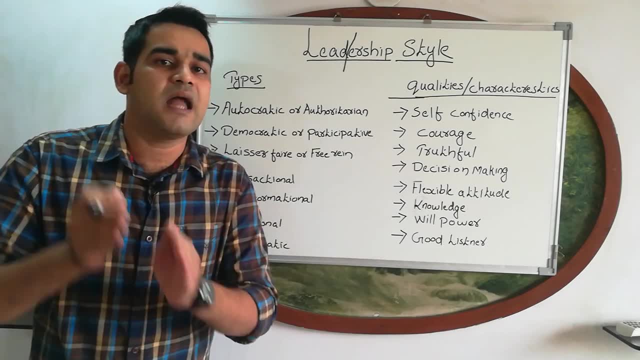 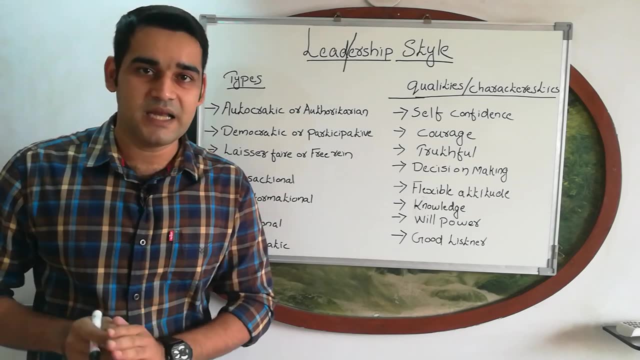 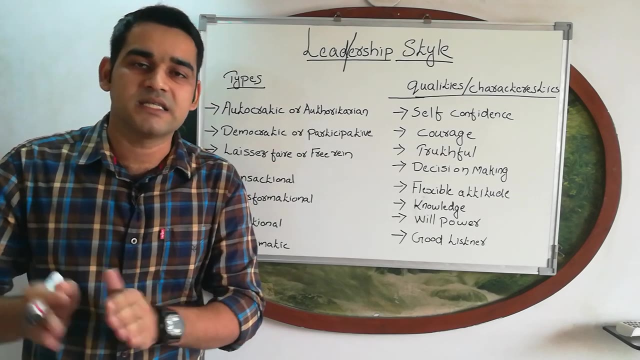 Okay, to achieve the goal, they will decide the thing and they will make the things together. only That is: we will decide and we will do. That is the difference between democratic and autocratic is: we will decide and we will do. That is the difference. 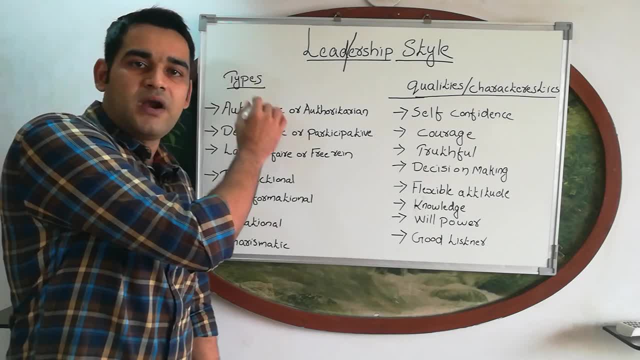 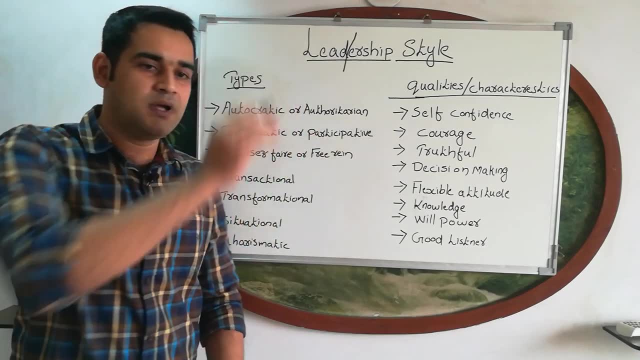 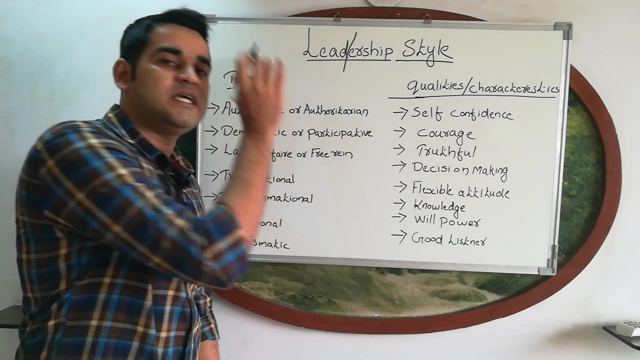 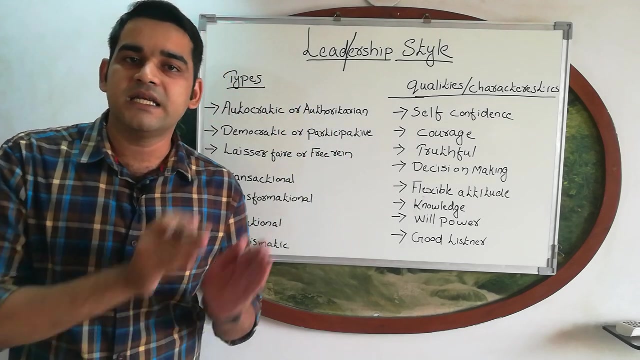 In autocratic means: I will order or I will decide and you should do, Okay. so here the participation of the workers are there in decision making and planning. That is called participative or democratic in nature. What is next. one is laissez-faire or free reign, or delegative leadership. 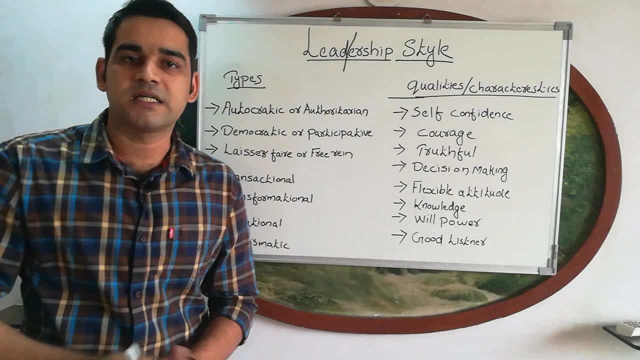 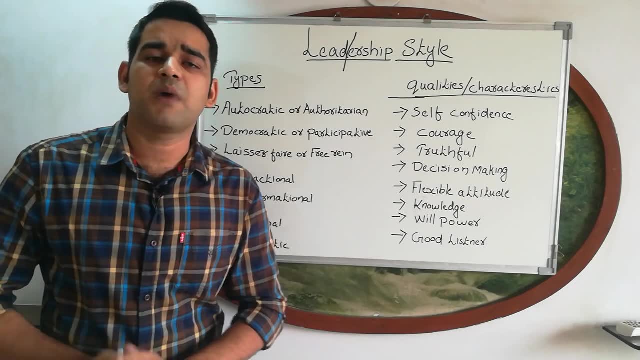 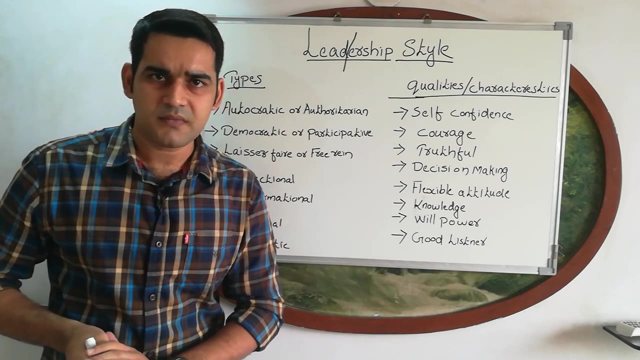 Laissez-faire or free reign leadership, or delegative, Delegative leadership. Okay, that means all the decisions are taken by the workers or the subordinates. All the decisions are taken by the workers or subordinates, But the responsible person is leader. 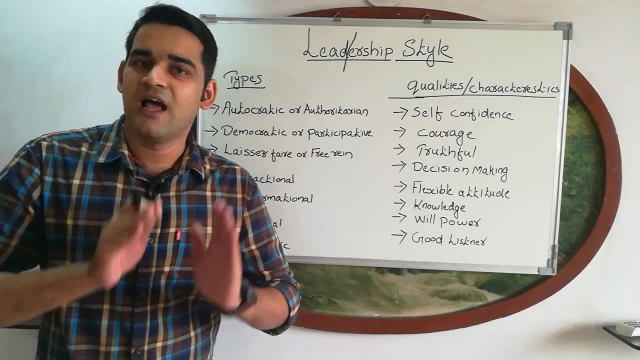 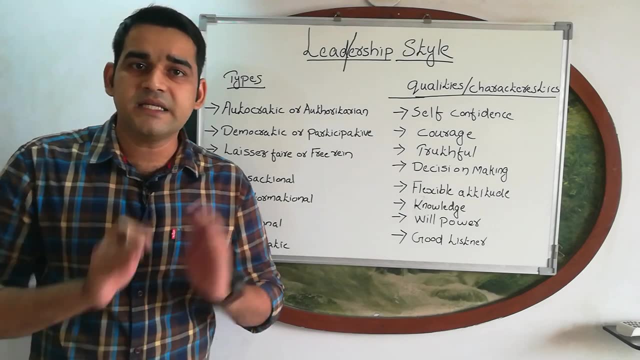 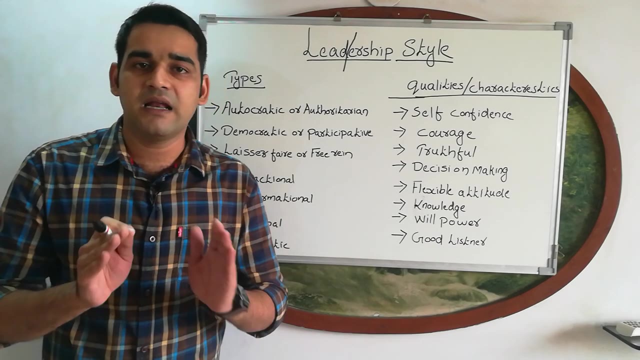 If anything has happened, the responsible person is leader only. Okay, but the decisions and plans are made by the workers only. This type of leadership is used when the subordinates- The subordinates or the workers are highly qualified and the leader has trust on them. 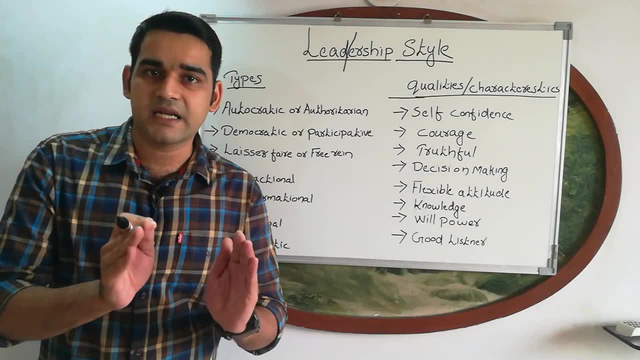 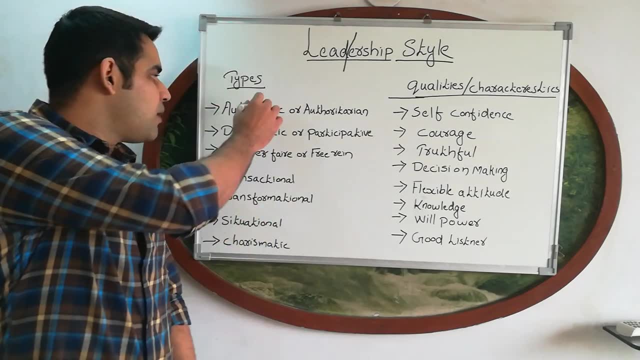 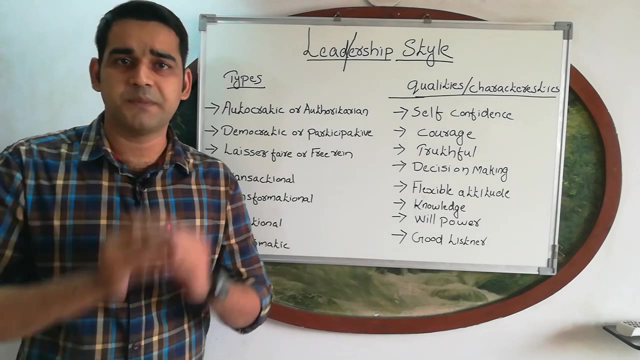 They will do it properly. So the leader will use this technique. that is, laissez-faire or free reign or delegative leadership. Got it. These are the most important or the main three types of leadership styles. Next we can see some other types of leadership styles. 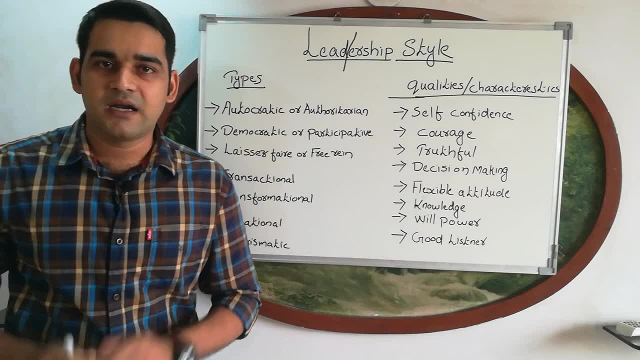 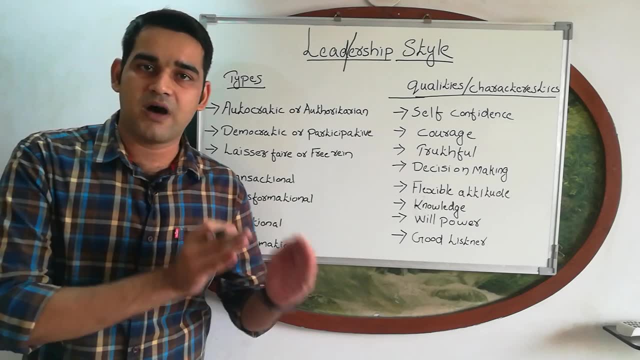 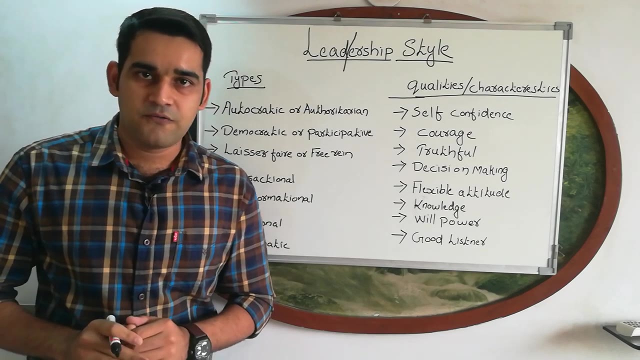 That is first. one is transactional leadership. Transactional leadership means The leader will divide the job. The leader will divide the work and he will distribute to the workers. For the good work he will give the reward. For the bad work he will give the punishment. 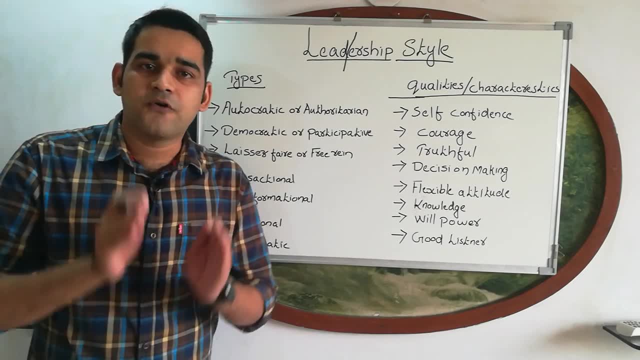 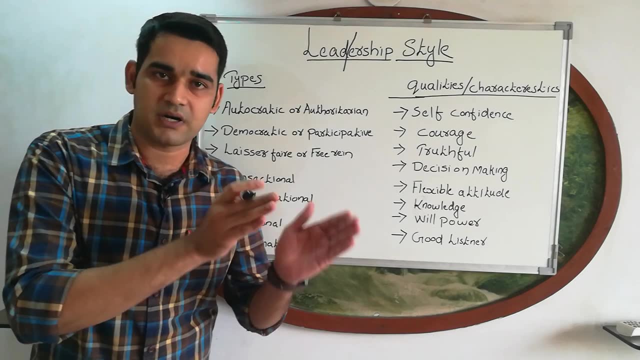 Okay, for the good work he will give the reward And for the bad work he will give the punishment. That is transactional. He will give the job to the workers and they should complete it properly. If they complete that work properly. 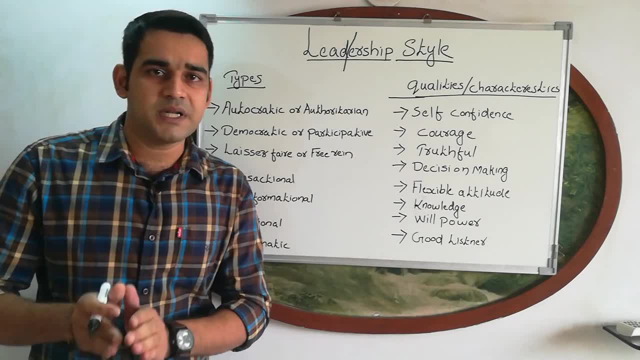 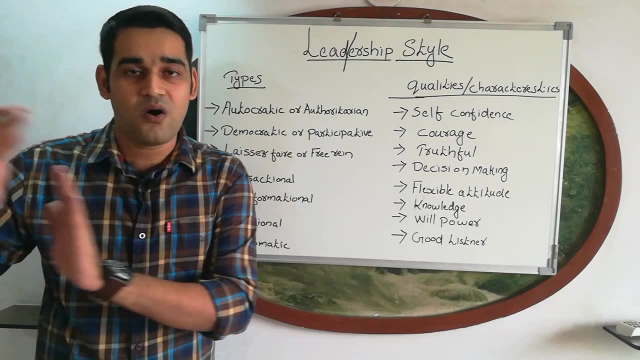 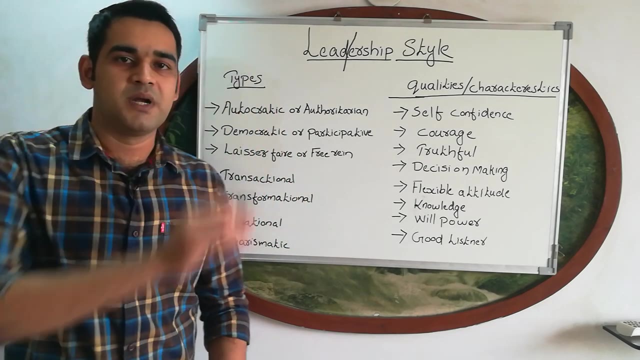 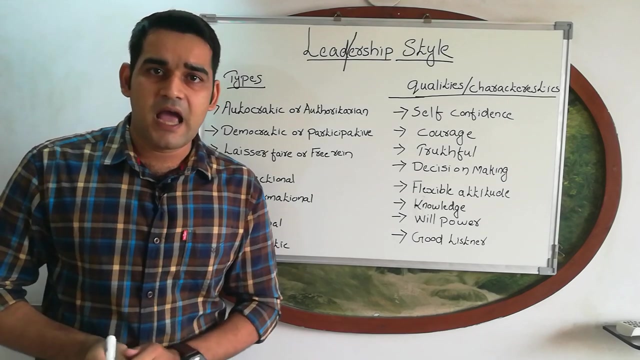 They will get a award. If they are not completed or if they go wrong, they will get punished. Okay, either reward or punishment. That is transactional leadership. Next one is transformational leadership. Transformational leadership means Here the leader will always encourage and he will care the employee and he will motivate the employee. 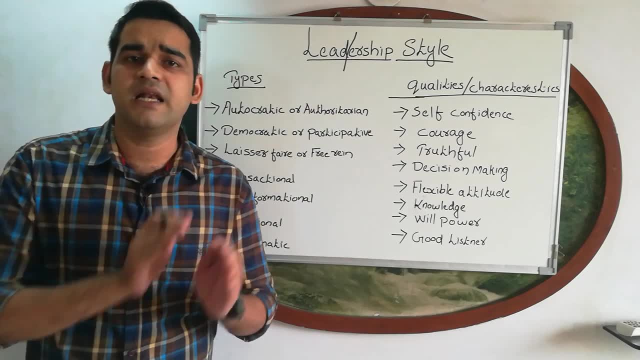 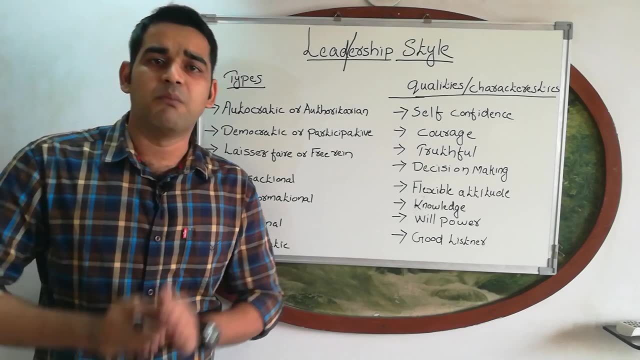 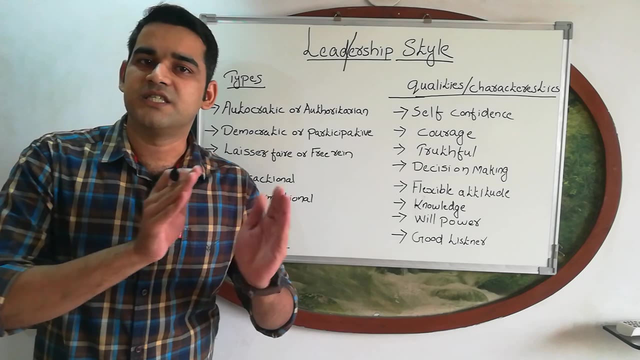 To achieve The goal. Okay, in transformational leadership, the leader will encourage always and he will care about the employee and he will motivate the employee to achieve the goal. Always he is caring and always he is encouraging and always the leader is motivating to achieve the common goal. 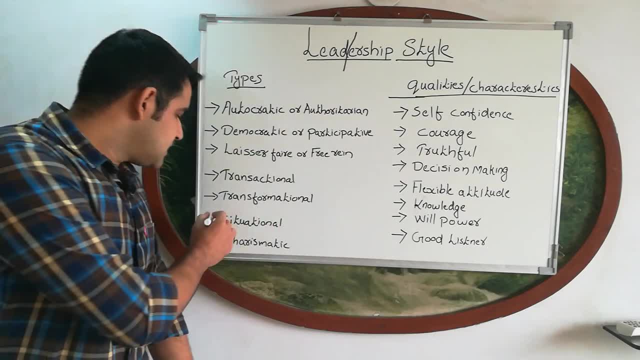 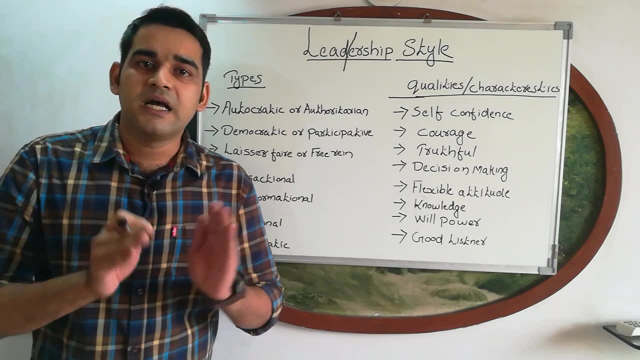 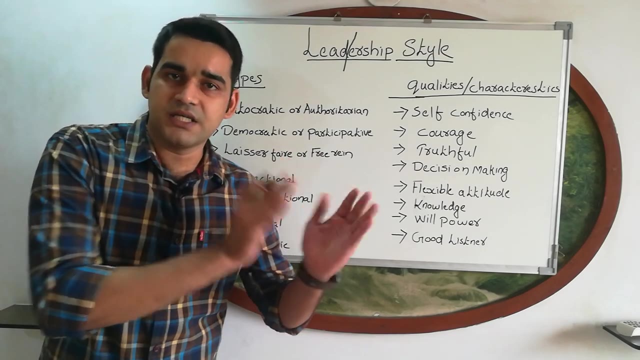 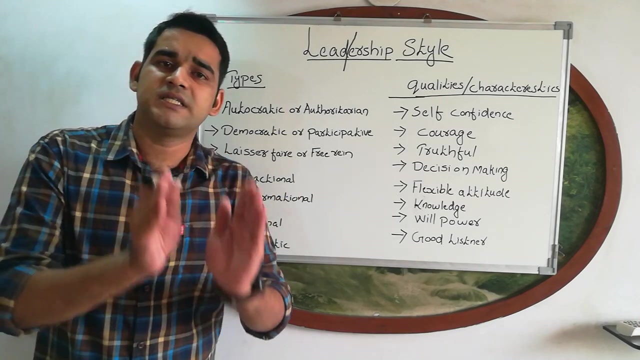 That is transformational leadership. Next one is situational leadership. Situational leadership means according to the situation, that decision May change. the leader will change the decision according to the situation Every time he is not using the same decision or same style. according to the situation, he will change the style. 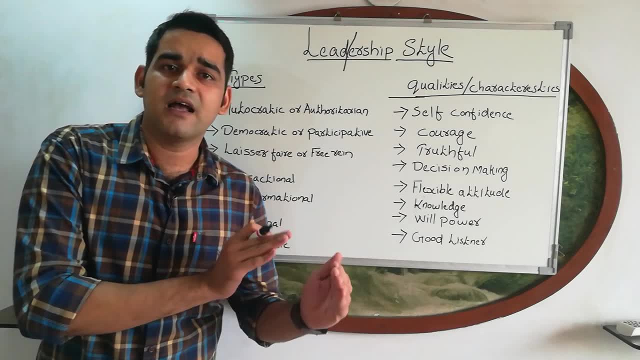 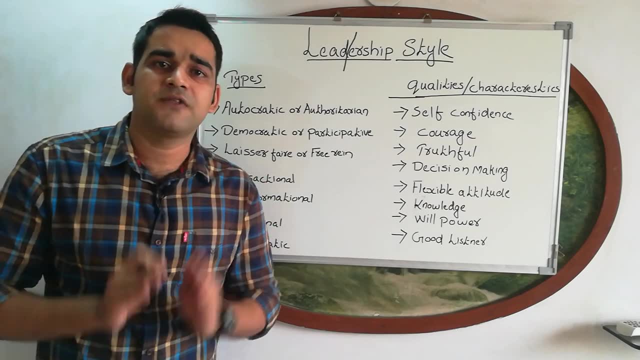 Okay. for example, according to the mood of the leader, the decision will change. or according to the mood of the workers, the decision may change. or according to the qualification: if the workers are freshers or they are new, the decision will be different. 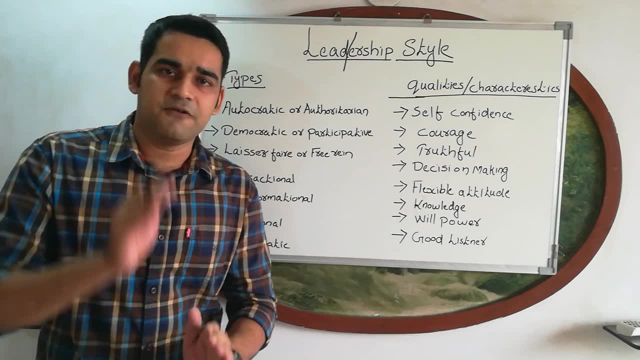 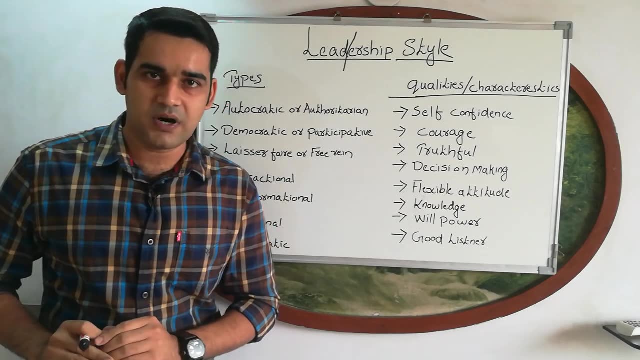 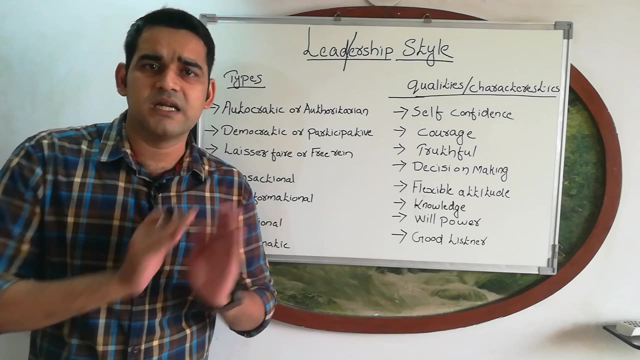 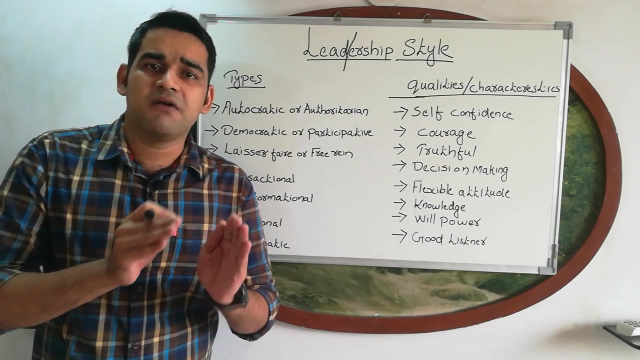 If the workers are Very experienced, the decision will be different. So according to the situation, the decision will change. That is situational leadership. What is next one is charismatic leadership. Charismatic leadership means very energetic leader. in charismatic leadership, Such leaders will be very energetic and they are very much influencing as well as they will have very good personality also. 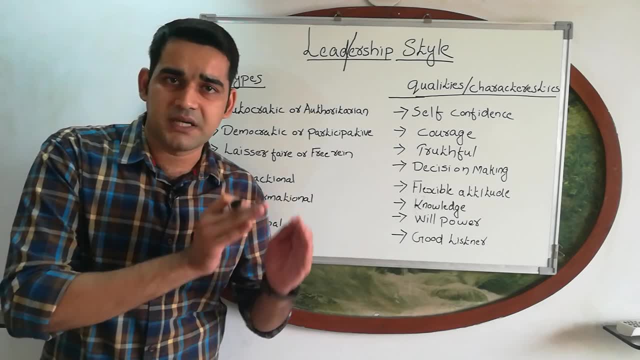 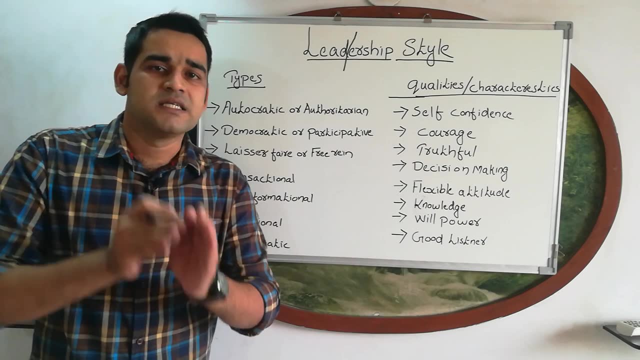 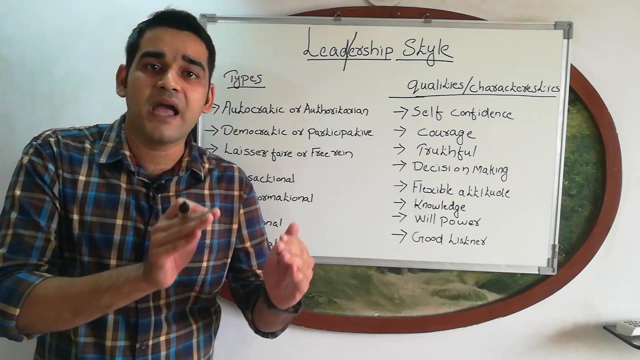 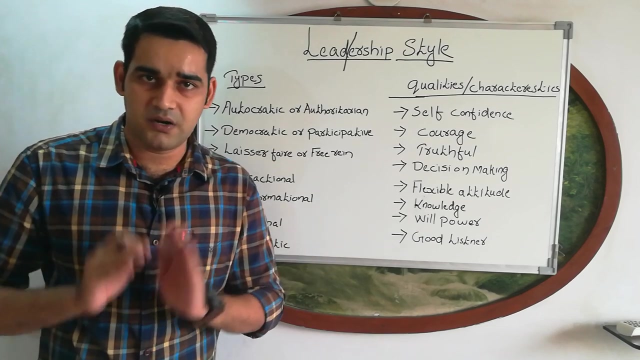 Okay and they are believing in their self Capacity. They will be very energetic, they will be having very good personality and they will be trust in their self capacity. People are follow him by his personality and by his action, Maybe in charismatic leadership. the leader will not have any power from the side of government, and all but his personality make him a good leader. 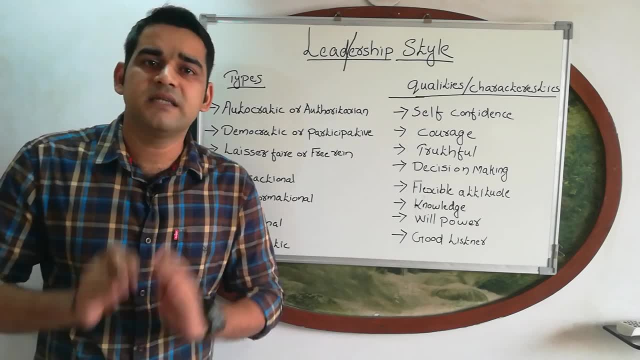 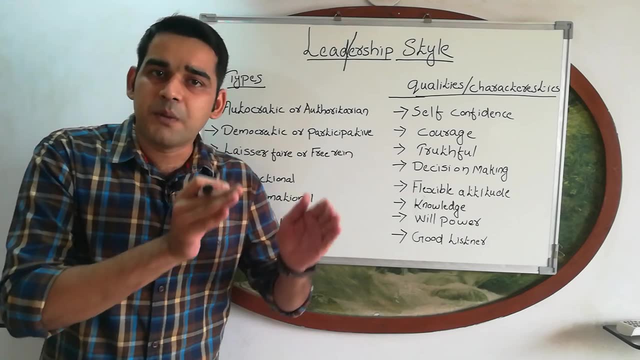 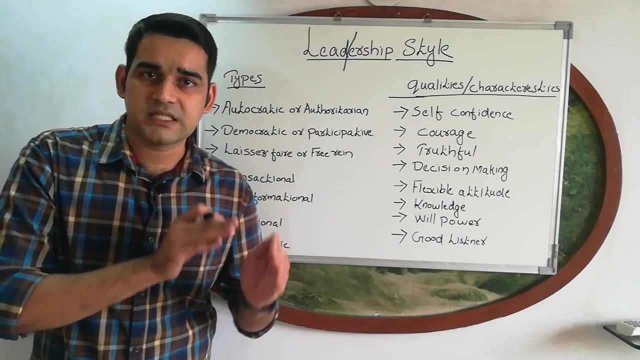 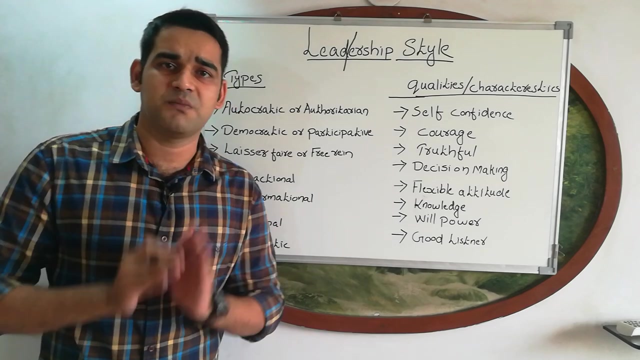 For example, you can take Mahatma Gandhi. Okay, He's a charismatic leader. from his energetic leadership and from his personality, People followed him. Okay, so that is charismatic leadership. He will be very much energetic and he is trust in his self capacity and he will have a good personality and he's influenced by taking his actions as well as he will be sacrifice. 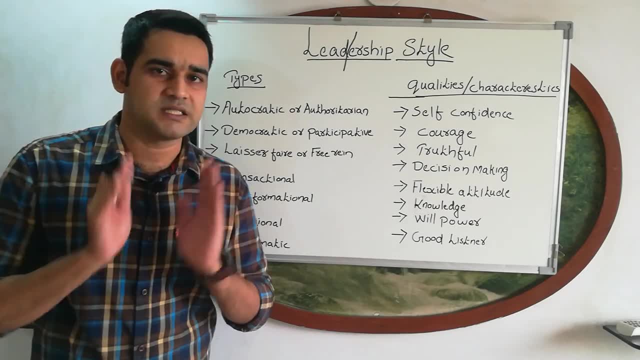 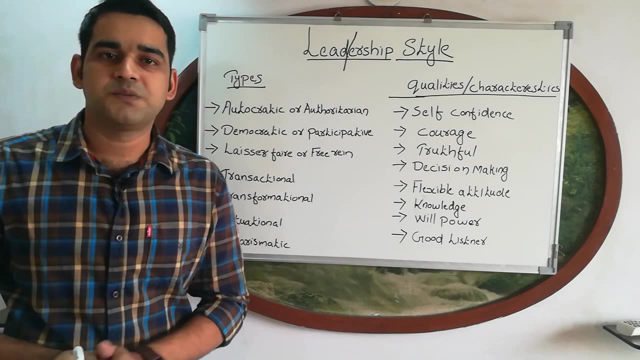 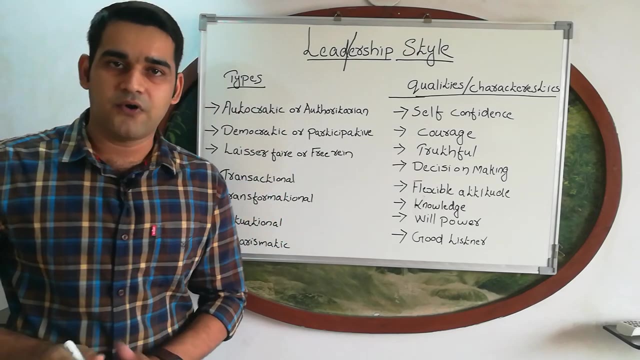 Also, he will do sacrifice also, So he will be very energetic. That is charismatic leadership style. Okay, that's all regarding the leadership styles- different leadership style We have discussed here. You can see some other leadership style also, but these are the most important one for you. 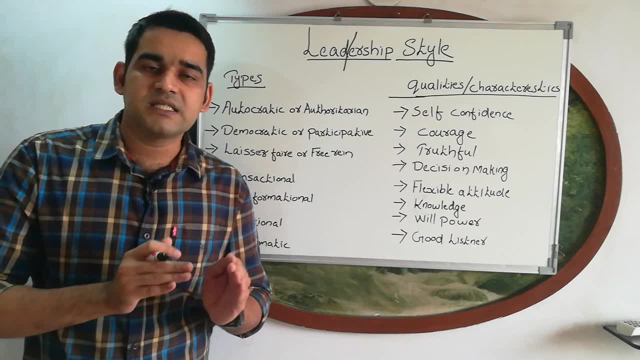 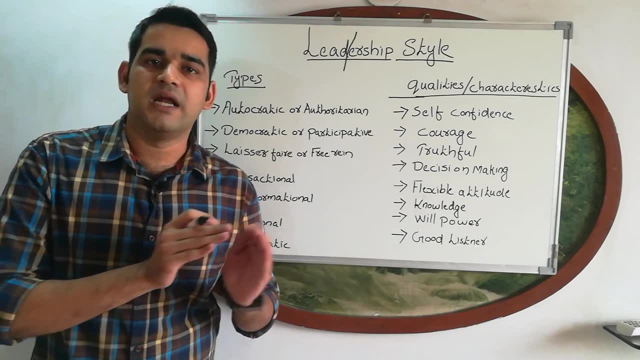 I have discussed here. Next we can see the qualities and characteristics of a good leader. What are the qualities or characteristics of a good leader? Maybe question may be asked like this also: qualities of a leader or characteristics of it. What are the qualities or characteristics of a good leader? 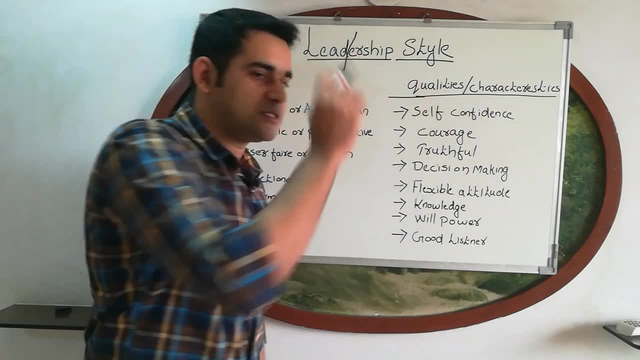 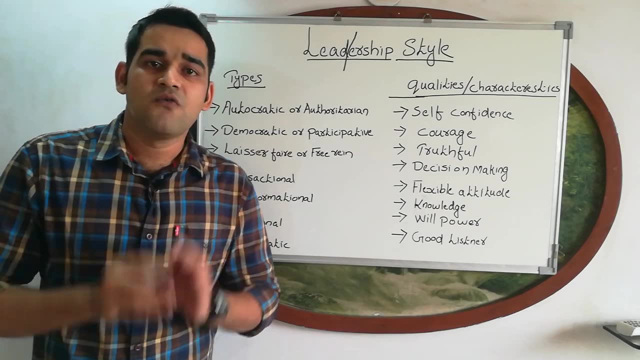 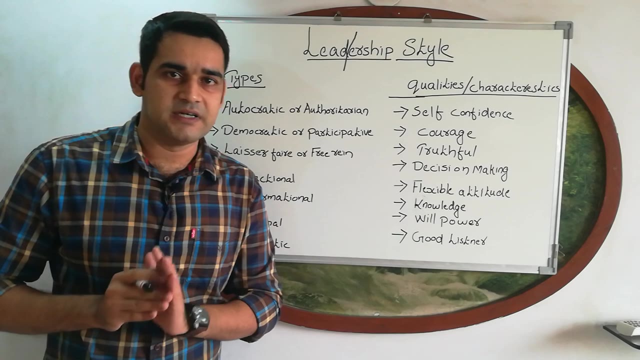 We can see one by one. First one is self-confidence. Self-confidence is the important quality of the leader. The leader should have self-confidence while taking any decision or while making any plan or while implementing any action. He should be self-confident. 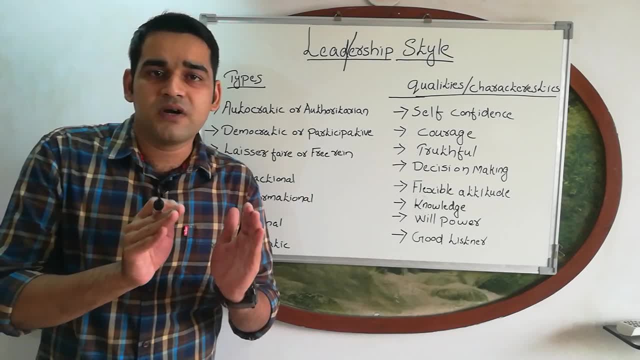 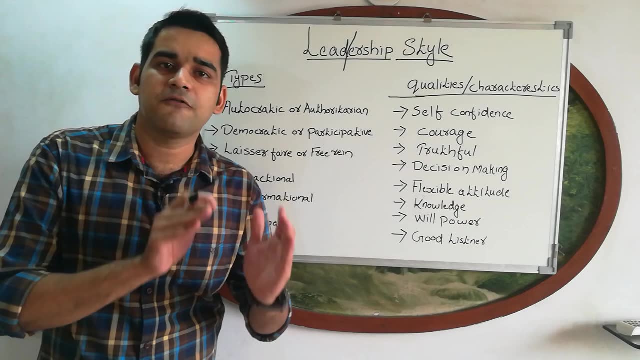 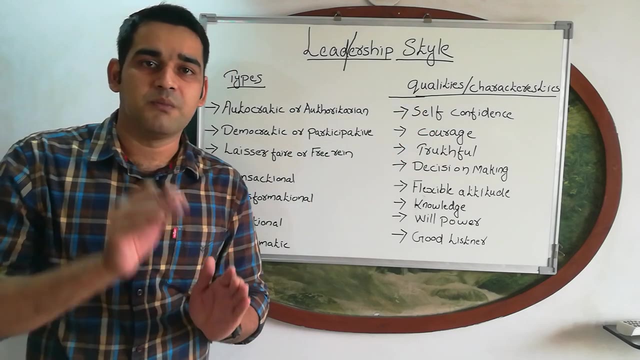 Okay, if confidence is not there means the followers will also get confused. Okay, so the main quality is self-confidence. should be there For a good leader. Okay, for example, you can elaborate it one by one. Okay, you can elaborate it one by one. 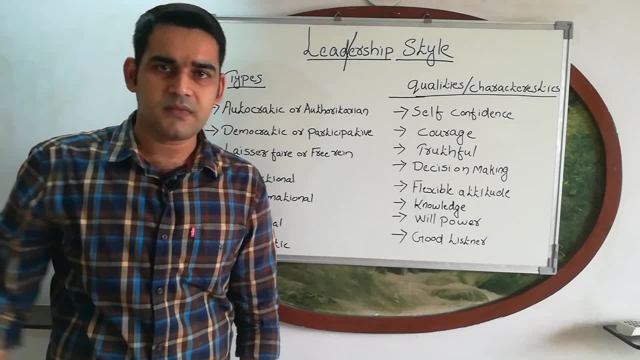 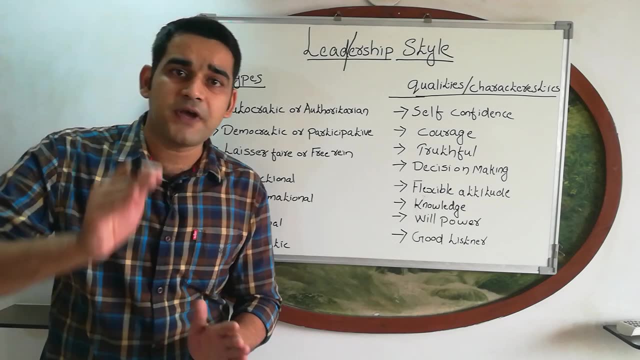 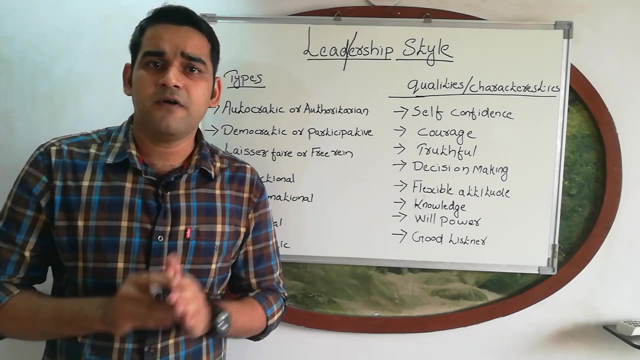 First one is self-confidence. Next one is courage. Courage means brave to take a decision or to solve a problem or to face a situation. Courage should be there. Okay, it should be a courage to face the situation. If fear is there means he can't take a proper decision. 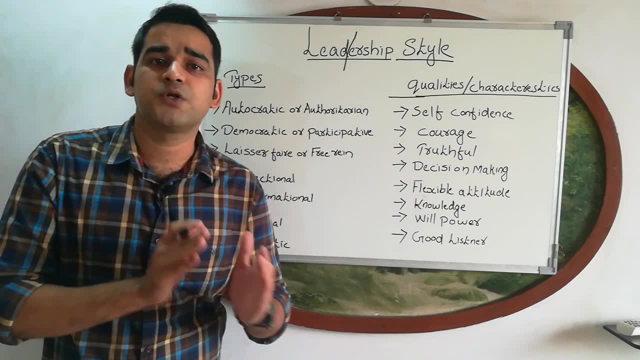 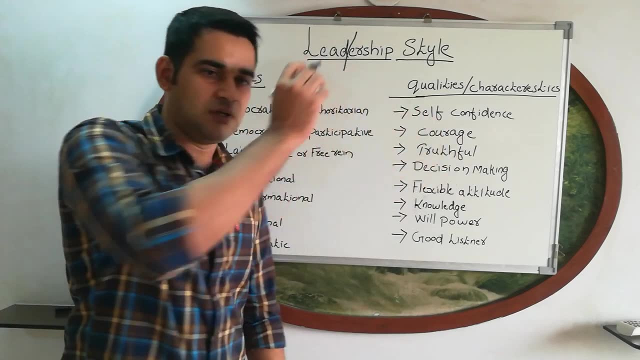 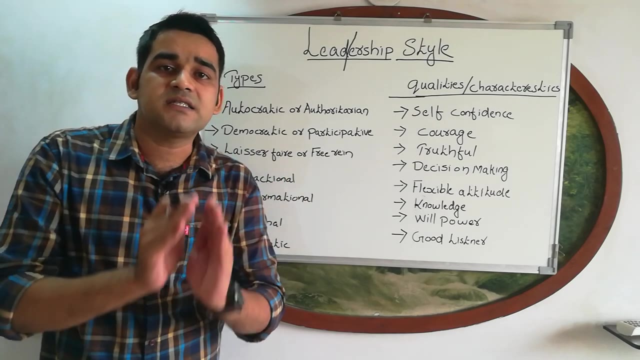 So courage- Courage should be there- or brave- The leader should be brave- to take the decision and to face the situation. That is courage. Next one is truthful. The leader should be always truthful. Then only he will build a trust relationship with the workers. 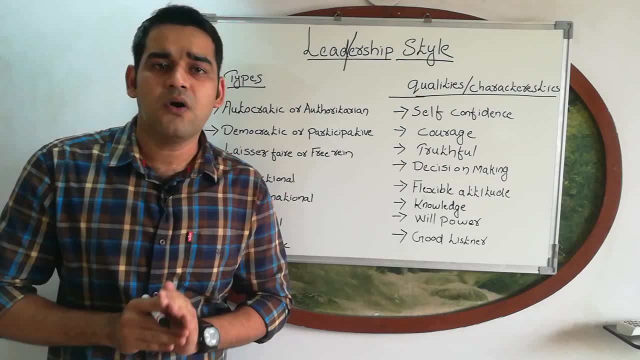 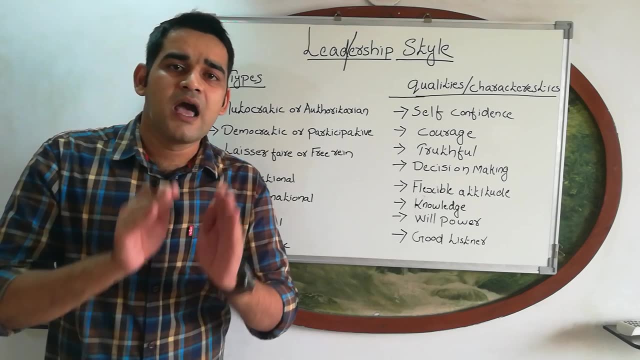 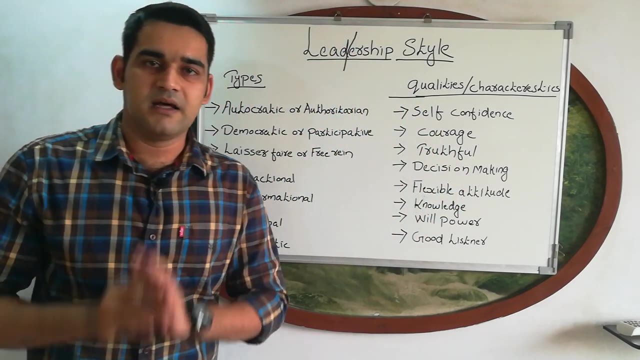 The workers should trust on the leader. So always the leader, a good leader, should be truthful. always, That is the quality or the character Characteristics of a leader is truthful. Next one is decision making. a good leader, or a good leader should be a good decision maker. 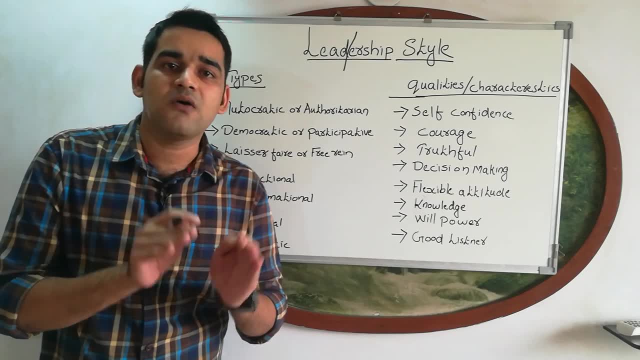 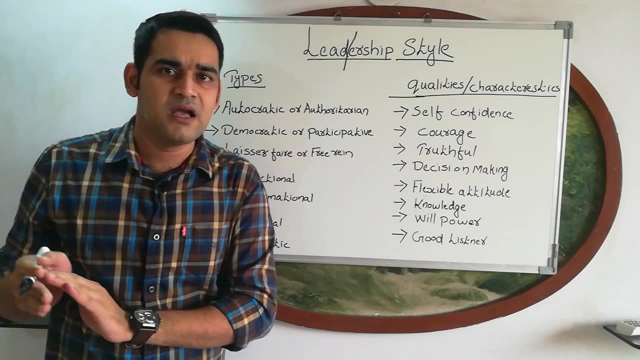 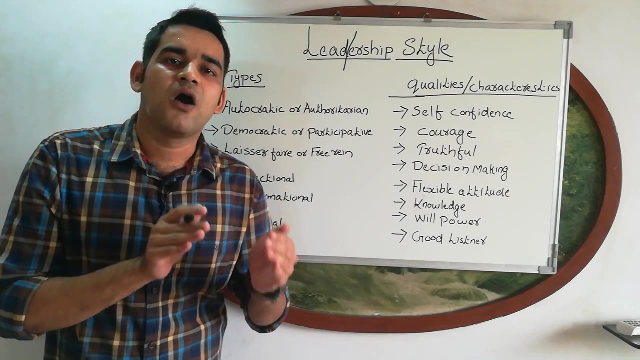 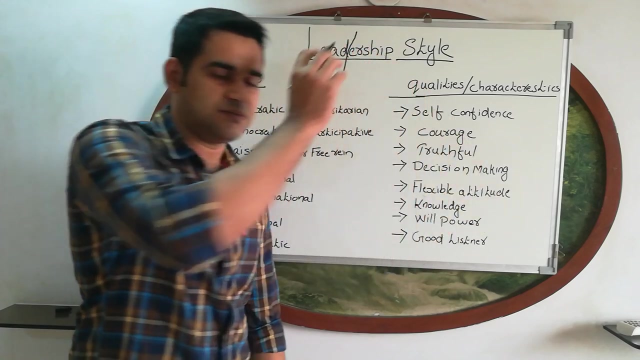 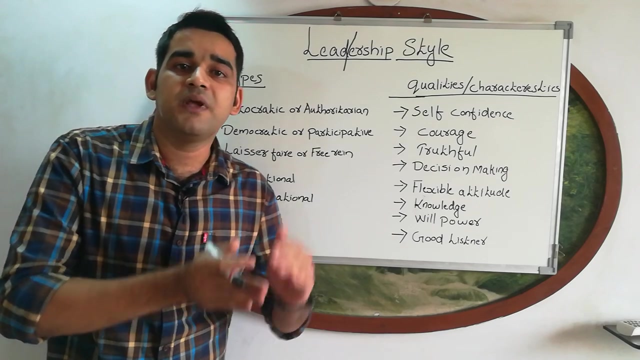 According to the situation, the decision making of the leader should be good. Okay. if a bad decision has taken, you can't call him as a good leader, Okay. so good decision is the quality, The quality of the good leader, but it next one is flexible attitude. flexible attitude means: according to the situation, the leader should be flexible. 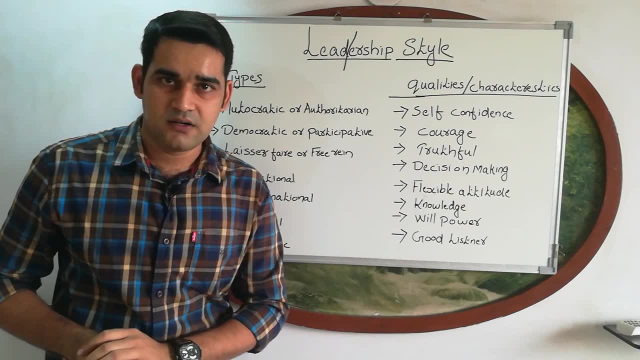 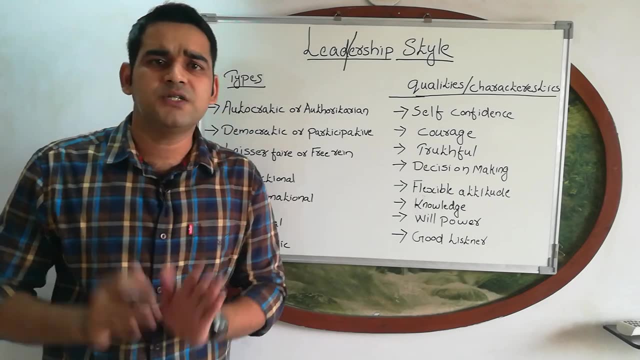 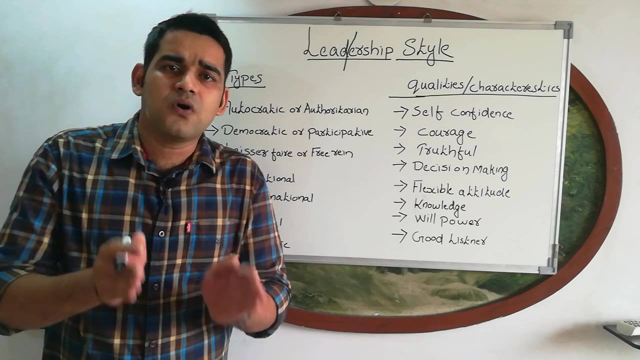 Suppose, if a problem is occurring in an organization, okay, electricity has gone and you have to complete that work, So we have to adapt another technique. He should be flexible according to the situation. Okay, So Workers are under strike. Okay, so he had to change his attitude according to the situation. 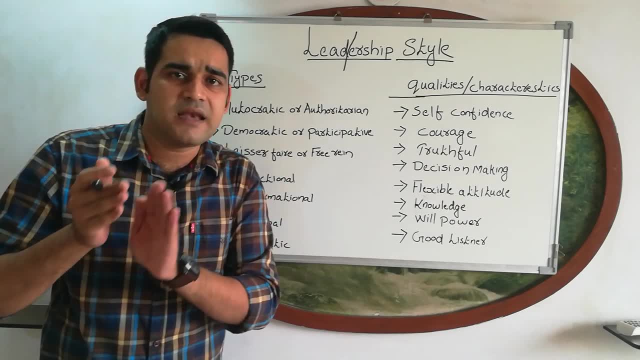 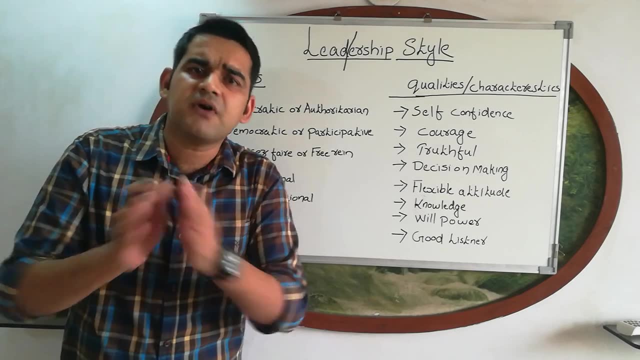 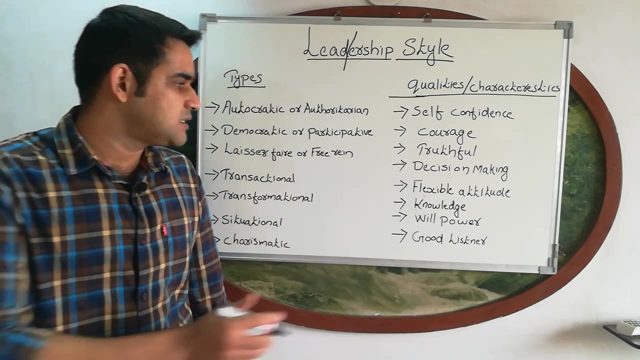 He had to be flexible. Okay, flexible attitude should be there. I will work like this. only in such condition Only I can perform, not like that. Whatever may be the condition, I will complete it. That is flexible attitude, Okay. next one is knowledge.